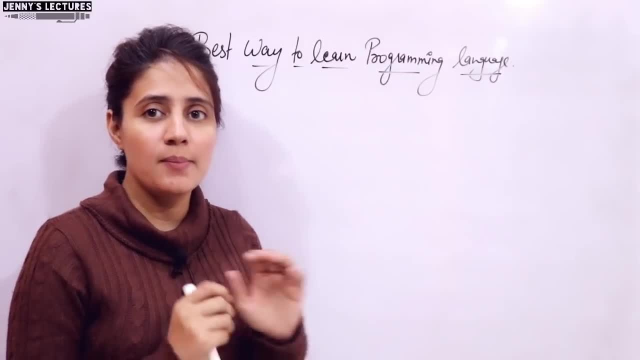 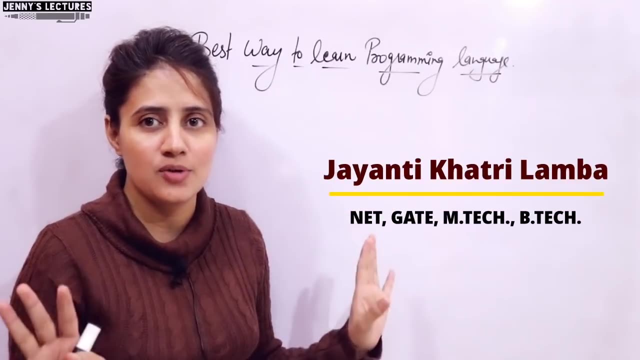 If you are thinking I am going to tell you any shortcut to learn a programming language, then this video is definitely for you. I am not going to tell you any shortcut, because there is no shortcut to learn a programming language. What I am going to tell you in this video is the right. 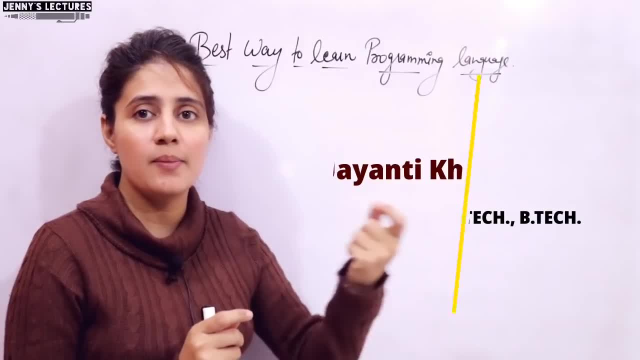 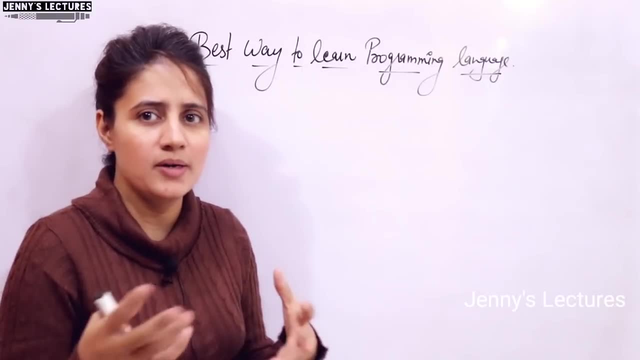 path to learn a programming language, best way to learn a programming language, what students do, how they learn a programming language. Maybe it's because of your- you know- college environment and that's the way they teach you. Like, in first semester you have C, you started learning C. 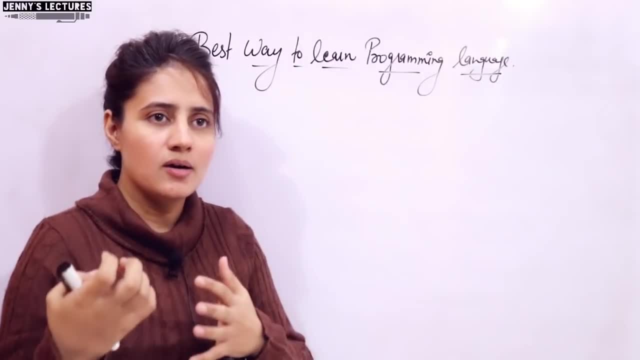 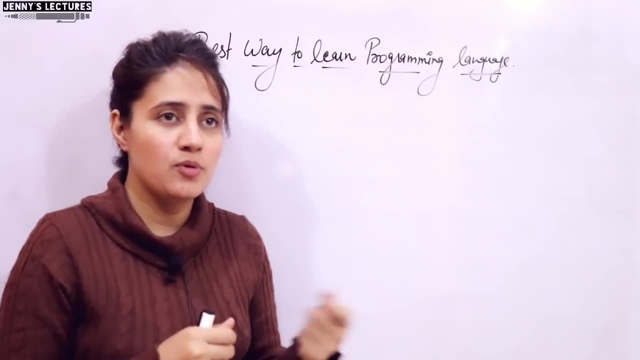 language. Like: first you will learn some syntaxes, then that hello world program, then some addition program, subtraction program, program to check whether a number is prime or not, whether number is even or odd, to find out factorial, to find out Febiniki series and some advanced level program. 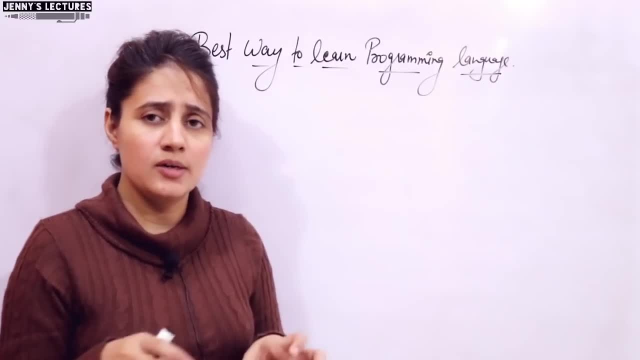 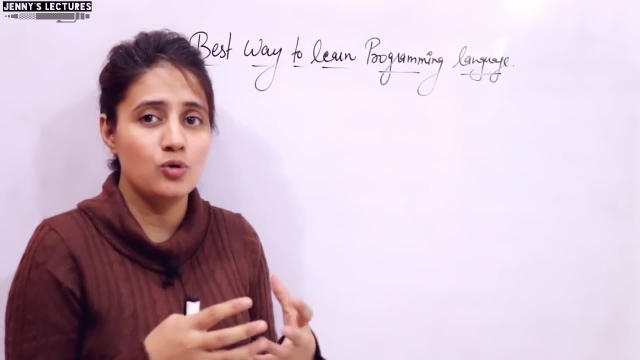 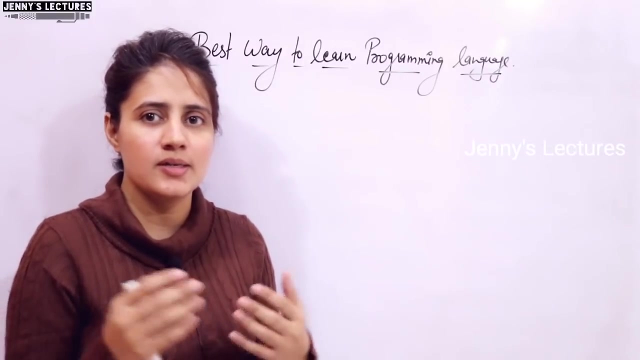 Right, that is how we exactly learn programming language. and then just your semester comes and- and most of the students do some ratification Also. I think they want to memorize those syntax, they want to memorize those programs just to pass the semester, so just to pass your lab practicals and that's over. In next semester you have C++. 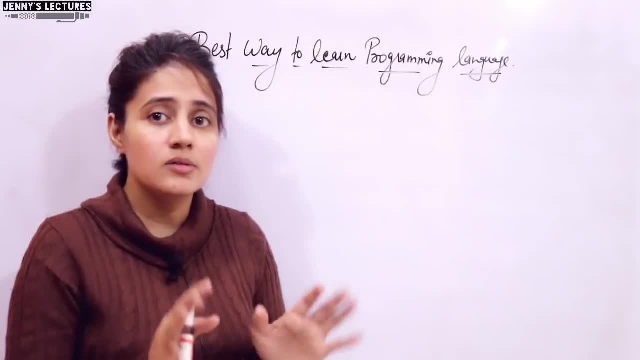 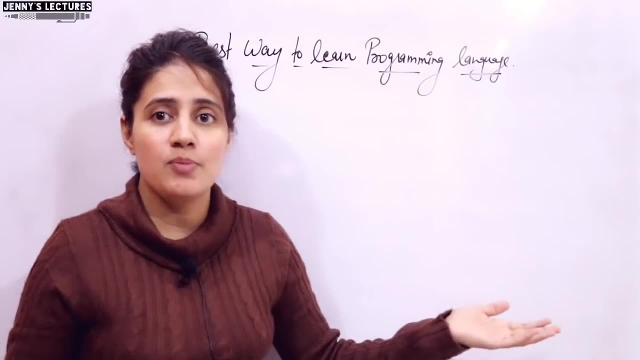 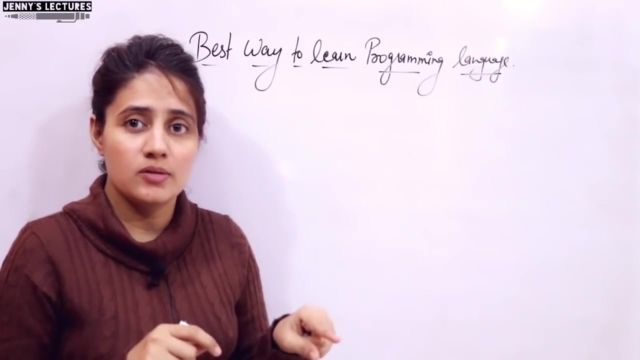 but see if you have written. sometimes many students think if you have written a program- hello world program- you have just printed hello world. and what? you think I am a programmer. No, you are not dear Right now. you don't even know P of programming. and if you follow this path, 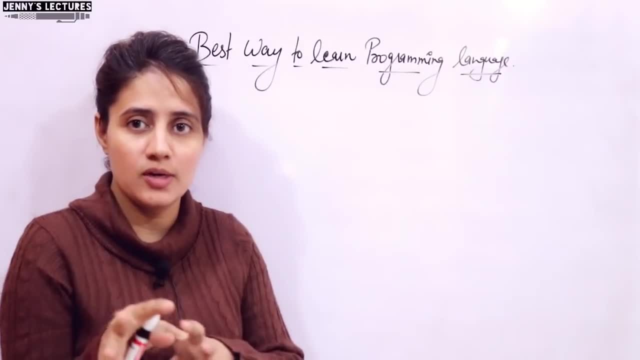 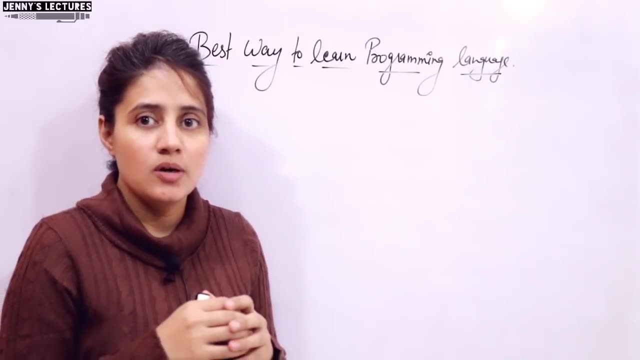 like this. you are not dear Right now. you don't even know P of programming and if you follow this I have discussed, that is going to be followed in your college. who learn a programming language at last. what you will say: I'm not good in implementing logic. I'm not able to think logic. I'm not. 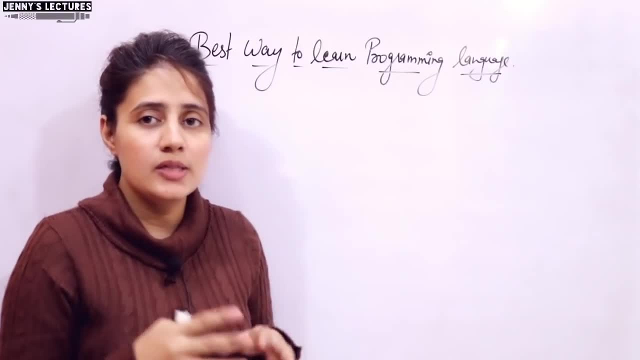 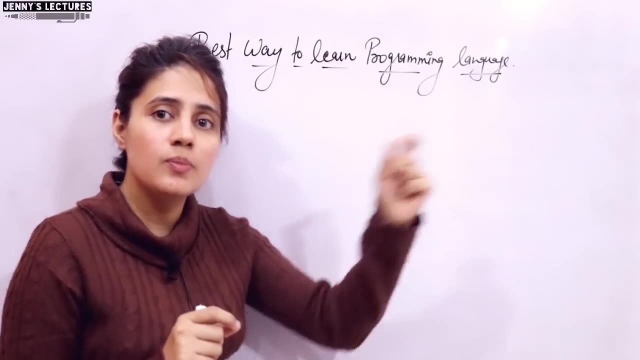 in. I'm not good in any programming language and ultimately, what you will think: it's very tough. I cannot learn any programming language, but the mistake is what, the path you follow to learn a programming language. It's not your mistake. you are right person. It's not like that Your. 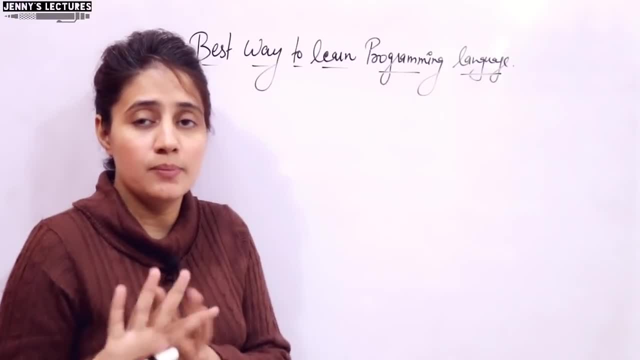 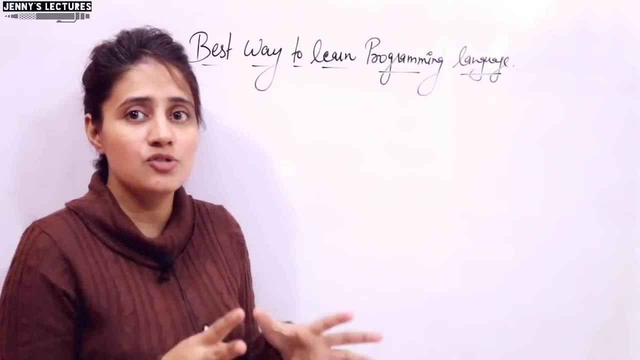 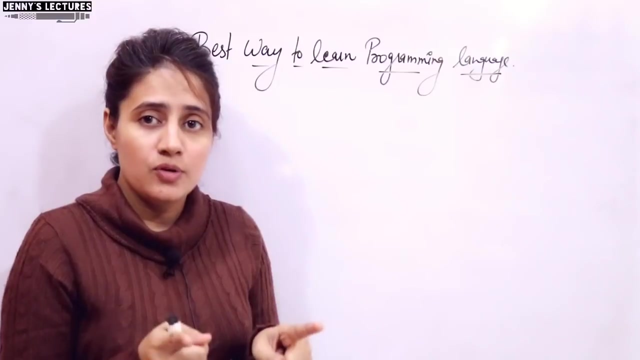 brain is not of that type, or you are a weak student, are dumb. no, the path you are following to learn a programming language that is wrong. so that's exactly i'm going to discuss in this video: the right path to learn a programming language. right before that, just want to tell you one thing: if you are interested in competitive programming, 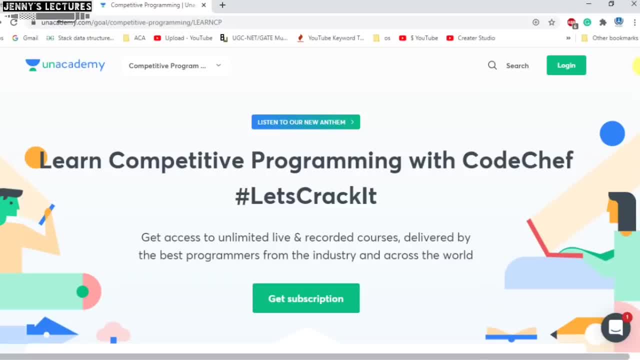 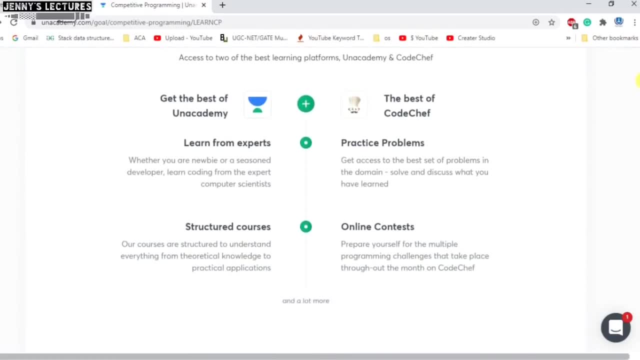 then anacademy, in collaboration with code chef, has started a course to learn competitive programming. there you can take free live classes. and if you are not able to take live classes, it's okay, you can attend their recorded sessions also. the top educators are going to teach you. those are. 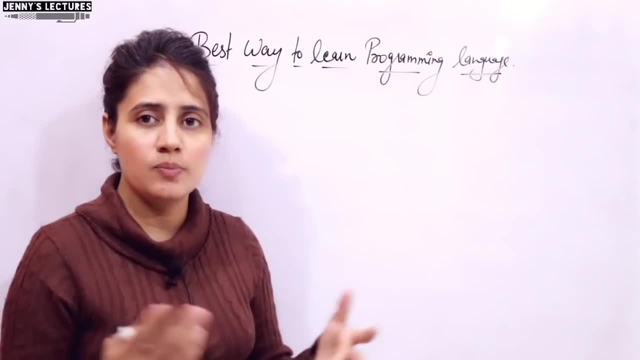 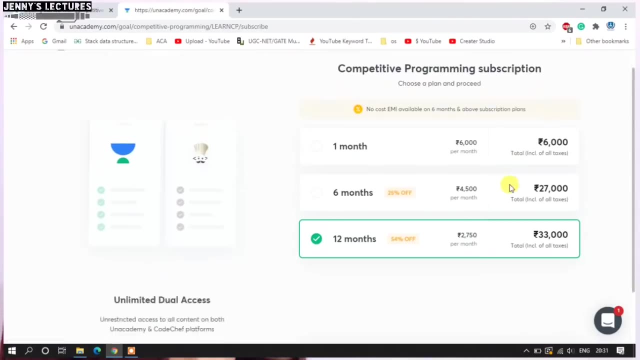 toppers of acm, icpc, finalist of icpc and working in top giant companies like google, flipkart, amazon, right, and if you like their free classes, then you can go for their paid subscription. and if you go for their paid subscription, after that you will get a proper structured course interactive. 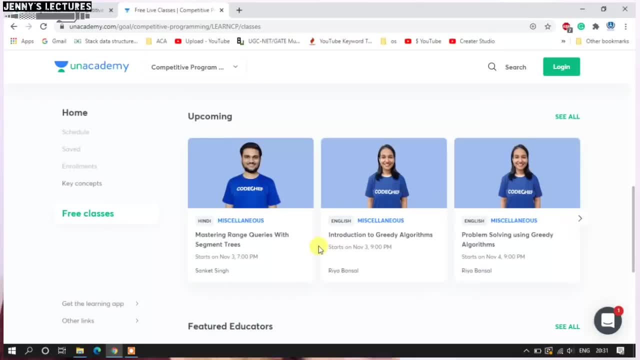 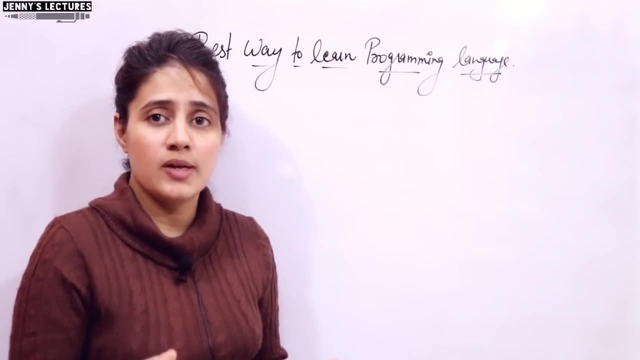 session would be there with these top educators. and one more thing: they have categorized these classes into three levels, like for beginners, for intermediate level and for educators- advanced level. so obviously you know yourself at what level you are in competitive programming. so according to that, you can watch that playlist. and these are free classes, so i will give. 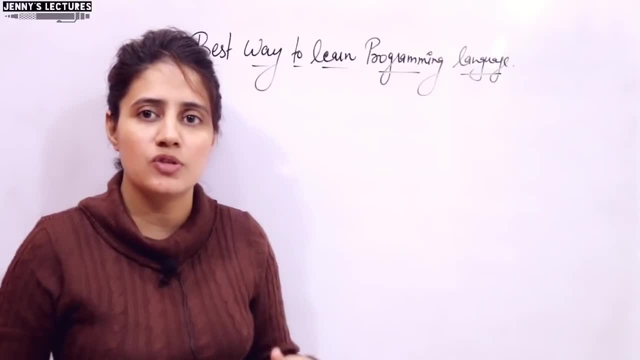 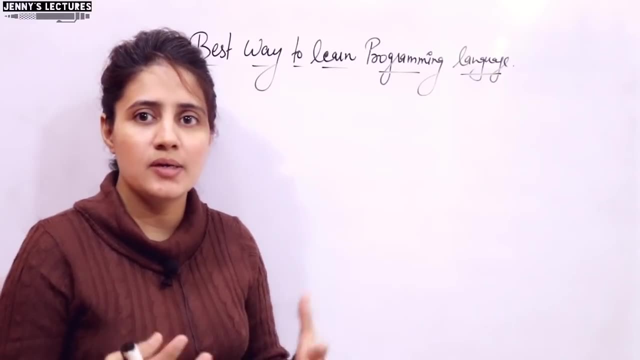 you the link of these free classes of all the levels in the description box of this video. you can go and check out. and a test is also there, like it's called a programming aptitude test, to test your programming skills. it is of 25 minutes and 10 mcqs would be there. 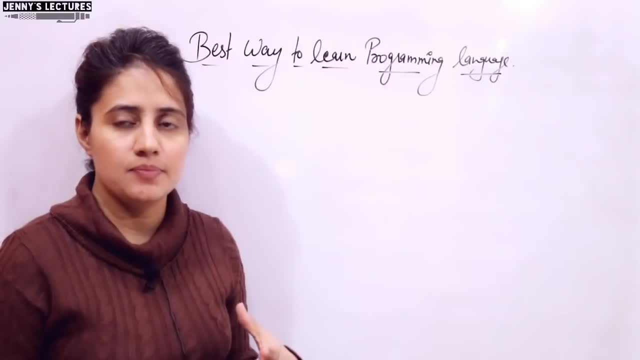 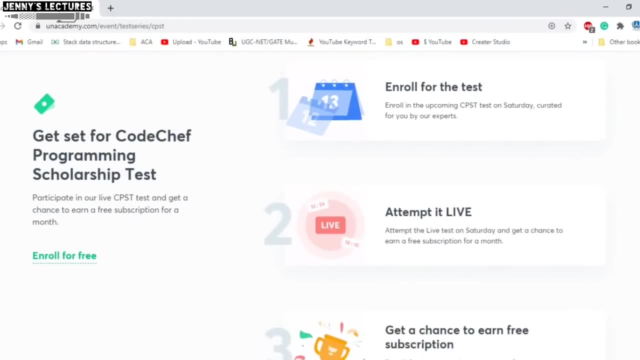 in this test. there is no validity of this test. you can take any time and they are also conducting a scholarship test named code chef programming scholarship test. that is on 12th of december and you can freely take this test. you just have to enroll, then you. 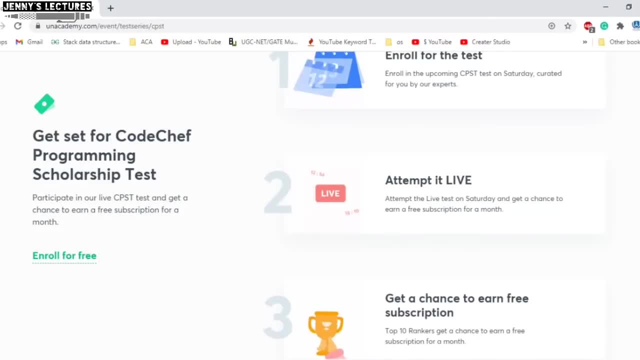 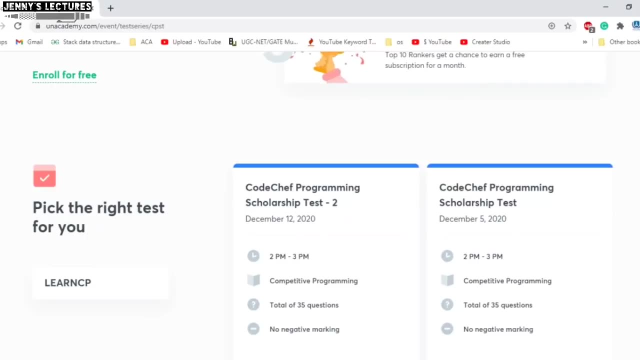 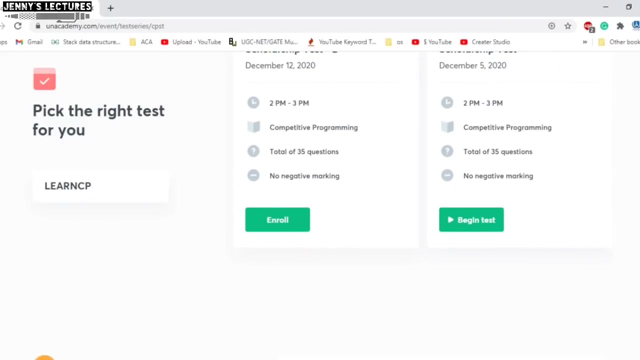 can attempt the test live and the top 10 rankers would get a chance to get a free subscription for one month. so you can pick the right test for you. the detail is over here, so if you are interested, you can go for these tests. all the links, whatever i have discussed here. 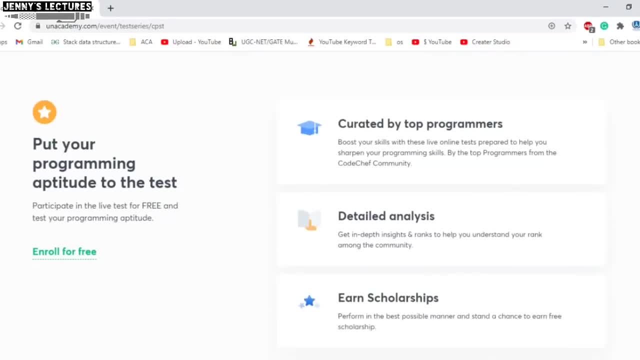 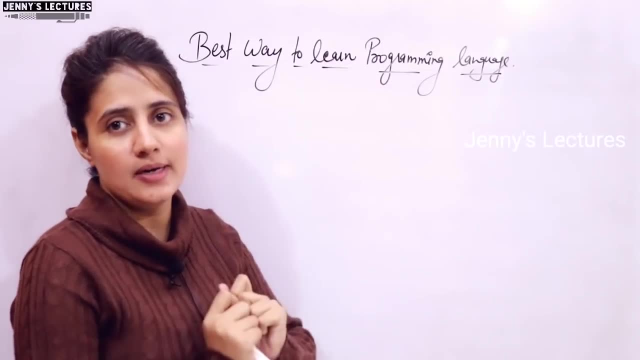 the links for those things i'll give you and all the details are in the description box i'll provide you in the description box of this video you can go and check out. so now let us discuss what is the right path, what is the best way to learn a programming language? 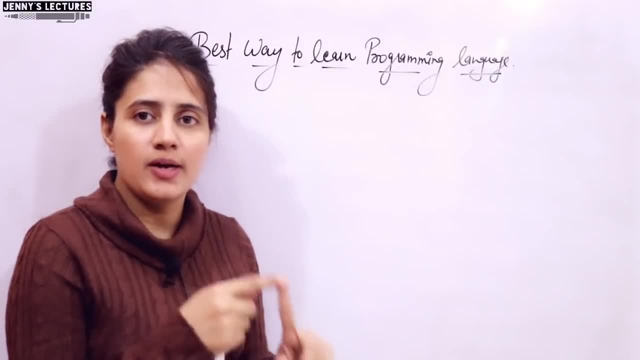 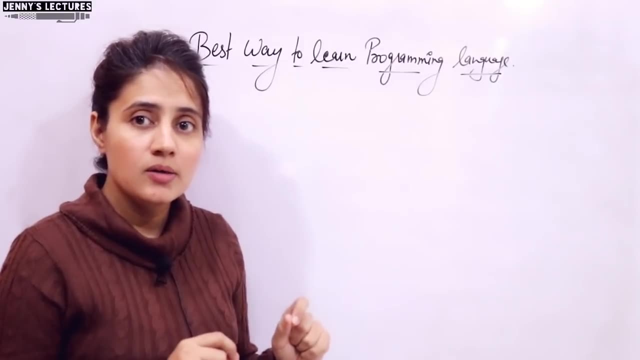 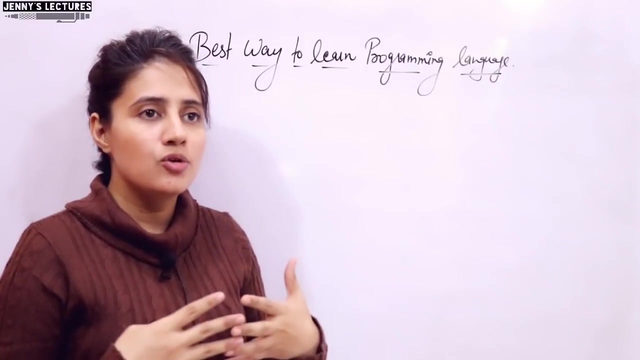 see. first point is very clear: you have to be good at fundamentals. so just pick one language in which you are interested: c, c plus plus, java, python, any language. pick one. clear your fundamentals. your fundamentals, your basics should be very strong, because if your basics are strong then it is, you know, very easy for you to grab the advanced concepts. and if your 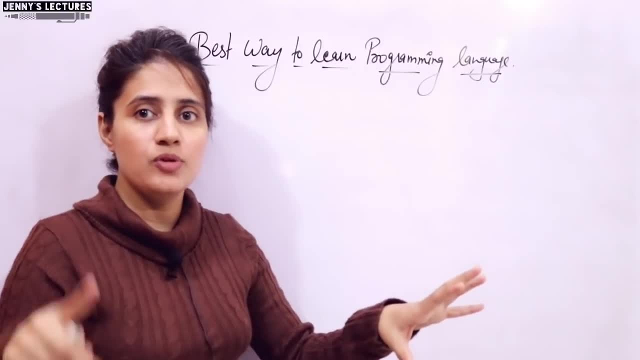 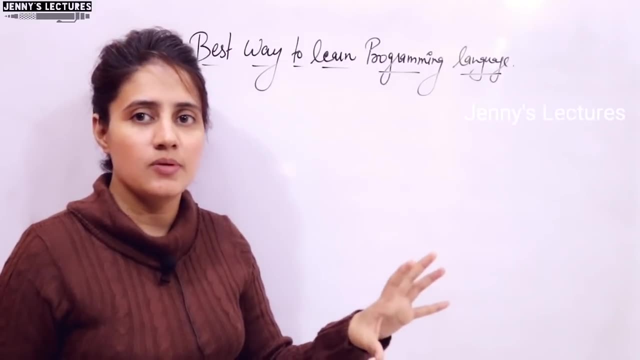 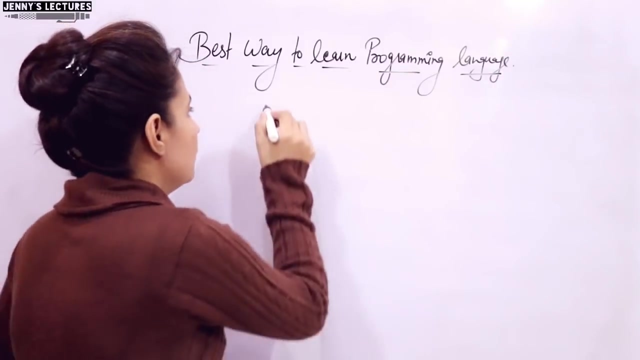 basics are not so strong and if you directly jump to the advanced topics, advanced concepts and definitely you will stuck somewhere. so first of all, work on your basics, right, that is very true. what you have to do next thing, after clearing your fundamentals, now what you have to do and see if you are learning a language by yourself, means you are not depending. 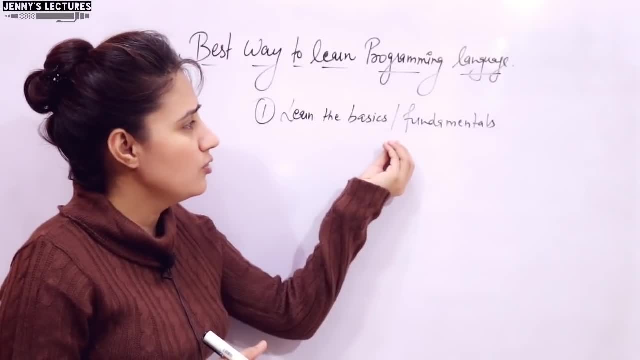 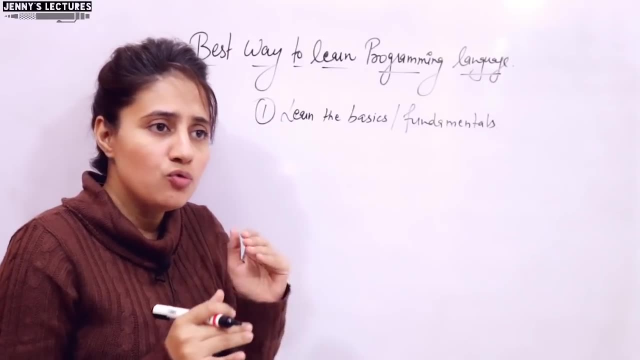 on whatever they teach in colleges so hardly. it will take five or ten days- maximum ten days- to learn fundamentals, to be good in fundamentals. after that you have to be good in fundamentals after that. it is not like that you have to complete the proper course of that c language. 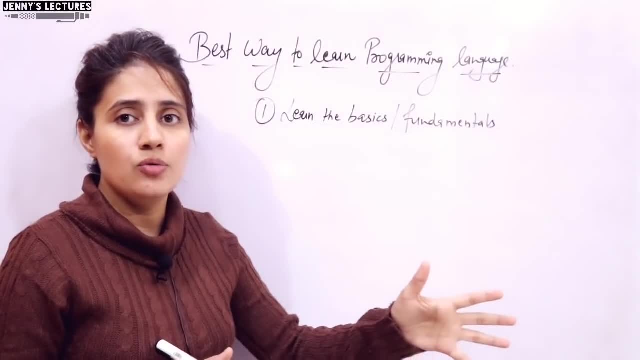 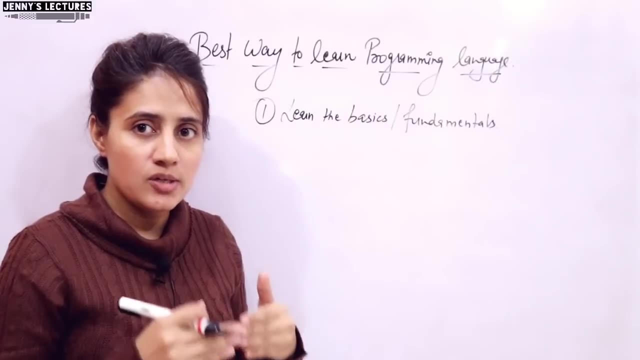 or any language you are choosing right now. what you have to do is second thing. what you have to do it is project based learning. you have to do now. it is time to pick a project, now it is time to work a project, to work on a project. right, maybe it is, if you are interested. 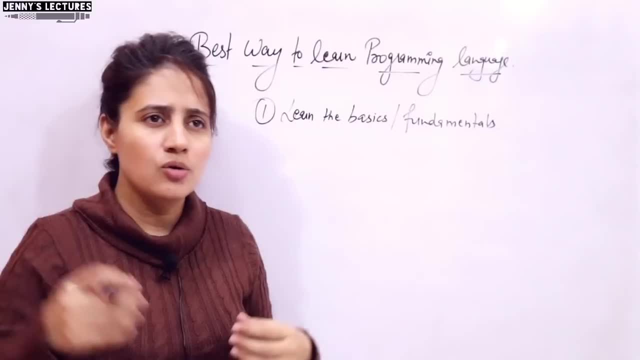 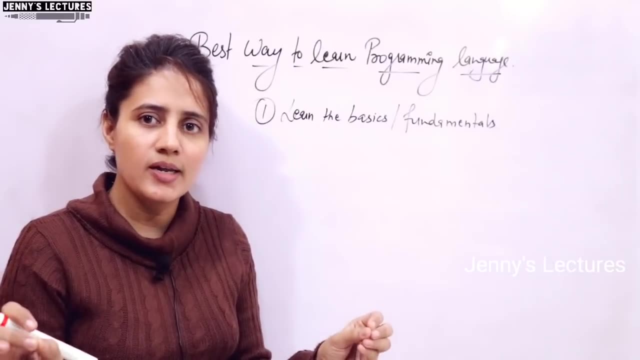 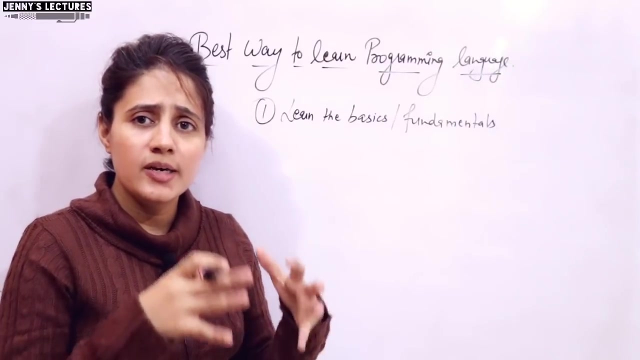 in any website development or any windows application or any app development, mobile app development, ios app development- take that project and then you have to complete the simple project, starting in starting. take simple project and start working on that project right. because see, whenever you are writing a program, like in in first semester, you have 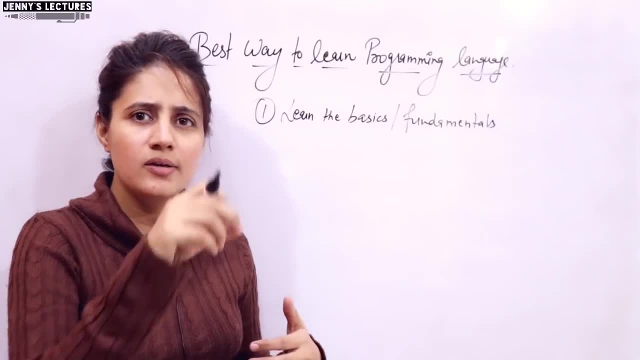 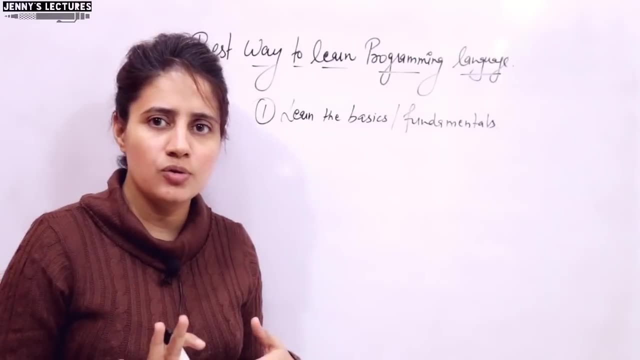 c language or in ah second semester you have c language. you are writing that programs, everything like to print hello world edition and to find out Fabiniki series and everything you are writing. it is okay, but now you know, do you know the, you know true meaning of writing those programs? or 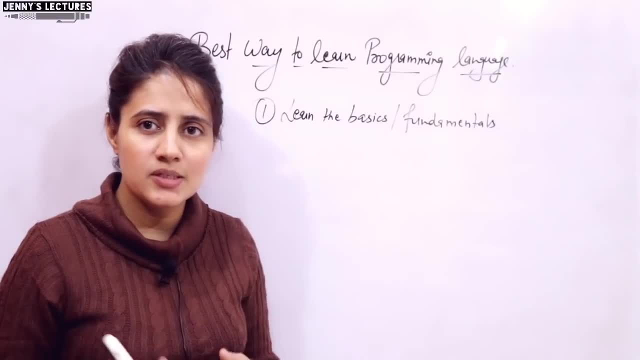 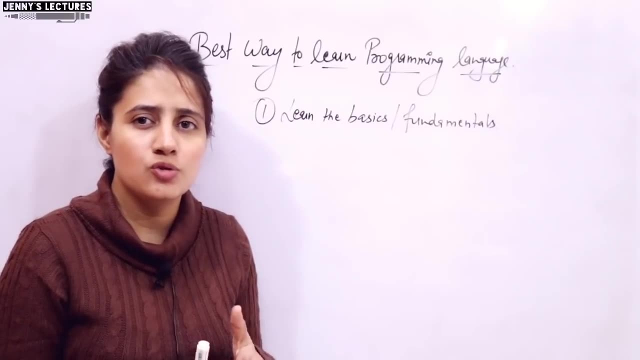 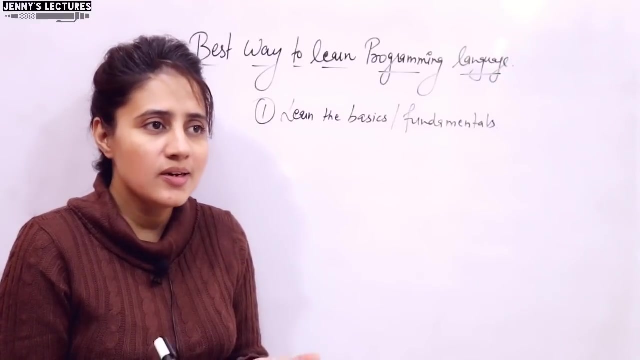 you are just writing programs, you are just learning that language to pass semester exams, to pass your lab practicals, that's it. i'm damn sure this question would have arised in mind of many students when they are learning any programming language, when they were writing code like why i'm writing this code, what is that? uh, that true. 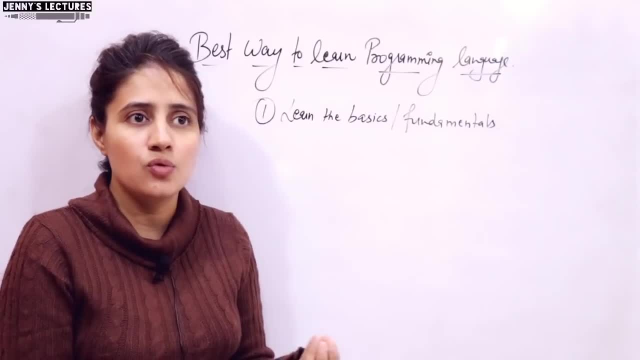 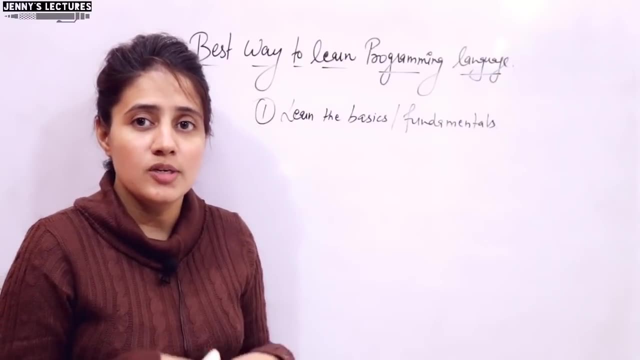 meaning of learning this programming language? what is the meaning of writing this for loop, where i will use this for loop or while loop or all the you know syntax or everything i'm learning here. so see, i'm going to tell you if you are playing a video game. behind that screen is also. 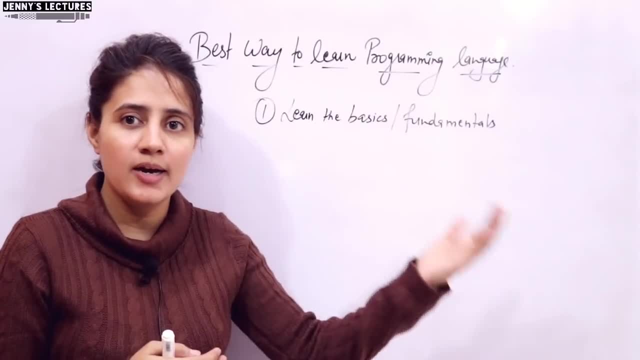 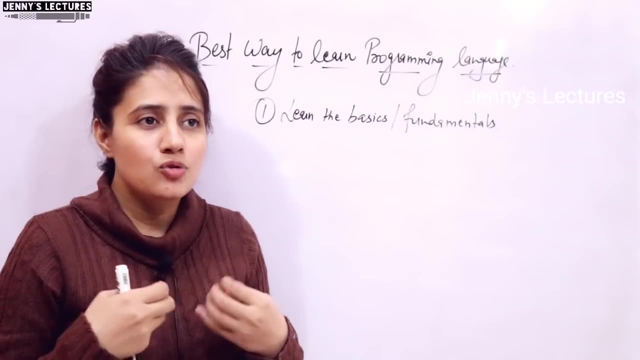 how you are able to play that video game. behind that, this is a software. behind that there is a lengthy code and someone has written that code. so i think why this programming language had been invented to: to make something, to build something so that people can use that thing to make some. 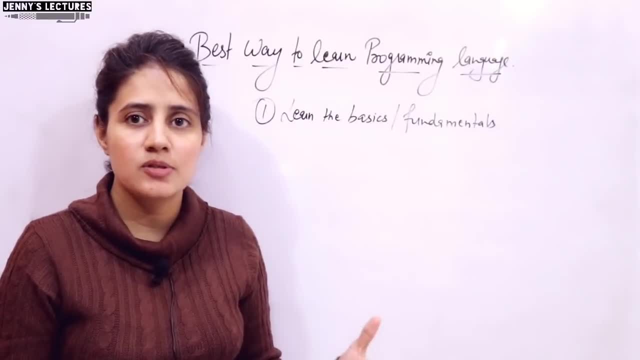 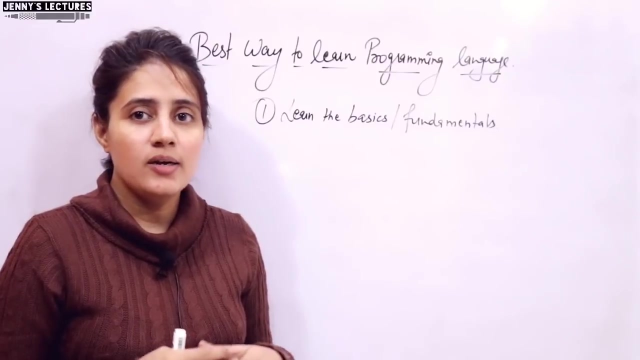 applications, some softwares, games or any apps, so that people can use those apps, those softwares, and it is going to make real life, the life of people, easy. they can use it. so i think that should be your reason: to learn a programming language, so that you can build something, so that you can. 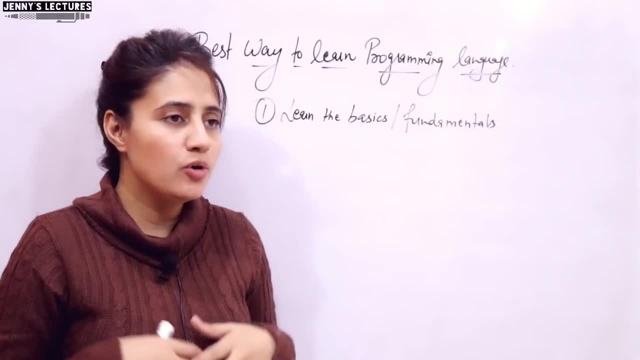 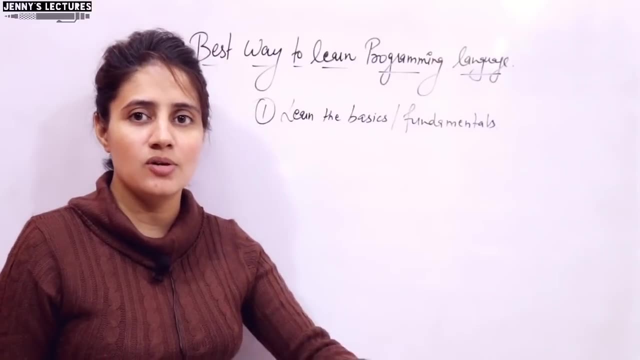 build any app or any software. any application people can use, it will going to make the life of others people easy. it is not like that. you are just learning a language because it's in your curriculum and you have to pass semester exam. you have to pass your practicals right, if you think. 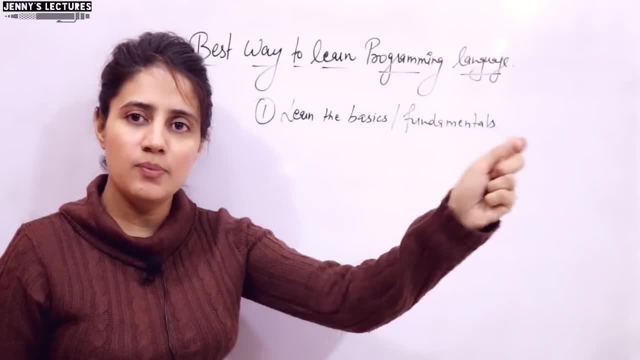 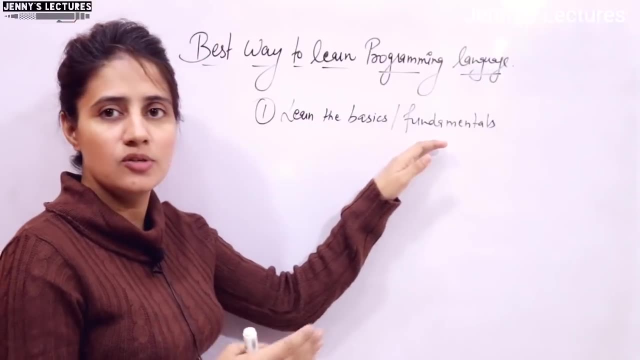 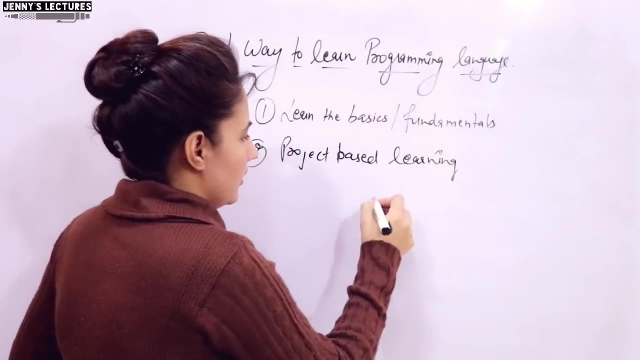 like this, then you will never be so good in a in any programming language. your aim should be to build something. so that's exactly: start working on a project after your fundamentals, after clearing your fundamentals, right, like suppose, if you are working on a project, maybe, uh, here, there, you want. 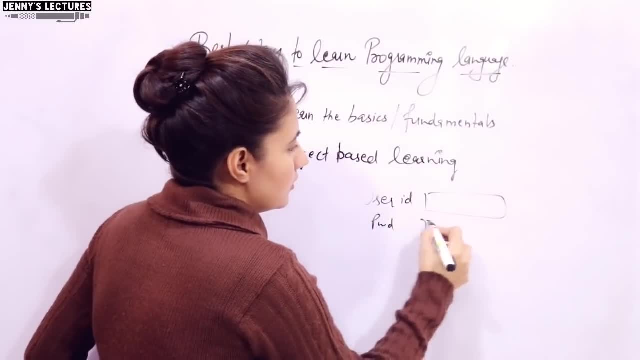 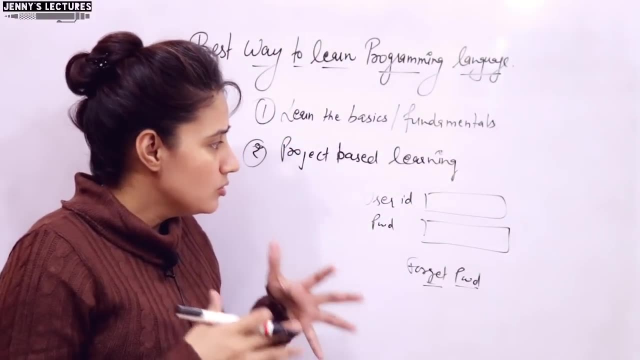 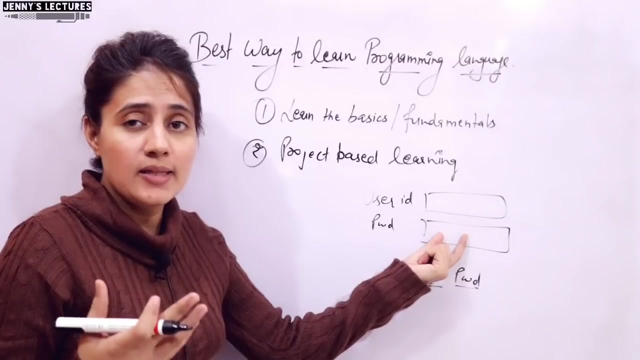 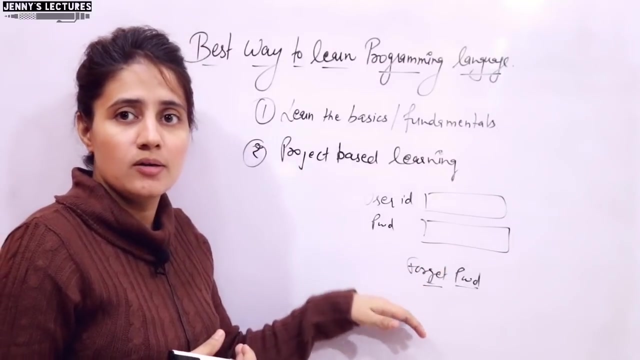 to implement, like user id and password, and then maybe forgot some kind of website you are you're making. so now you will, you know, search how you can make this text box and if in password, how you can- uh, you know, uh- apply that validation, like if someone enter wrong user id, wrong password, then it is definitely. it should show that you have. 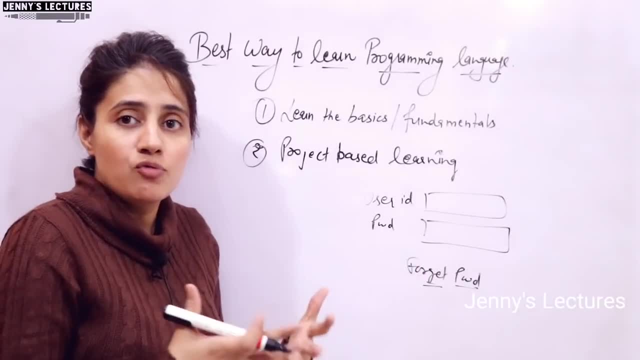 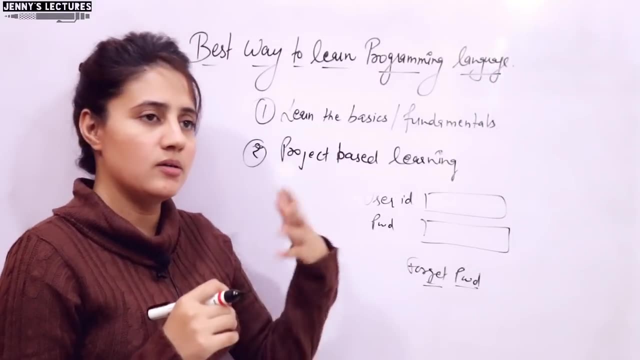 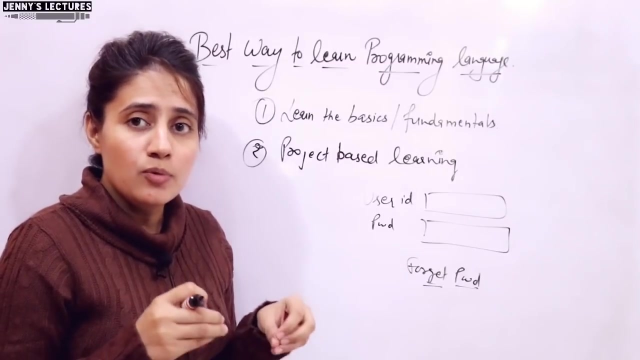 entered incorrect user id or incorrect password, right. so how to implement this logic? then you will search, you can ask help for others, like many platforms are also there, like stack overflow or many platforms are there. there you can post your question. you will definitely get a good answer. then you will come to know the true meaning why you are learning everything that in. 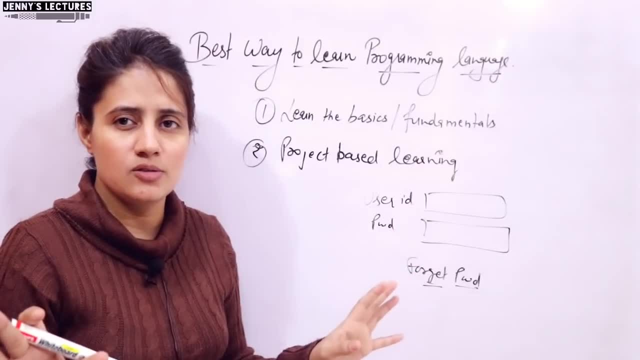 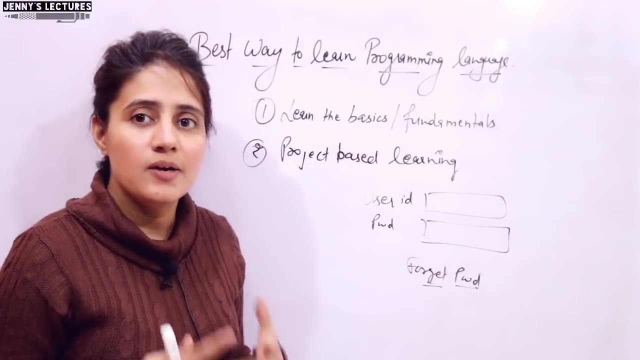 programming language for loops and everything like any other things also, like: yeah, this is how we are going to check validation. okay, this is the code. that is why i am using this, so better to start playing with code as early as possible. it's kind of active learning rather than passive learning, and 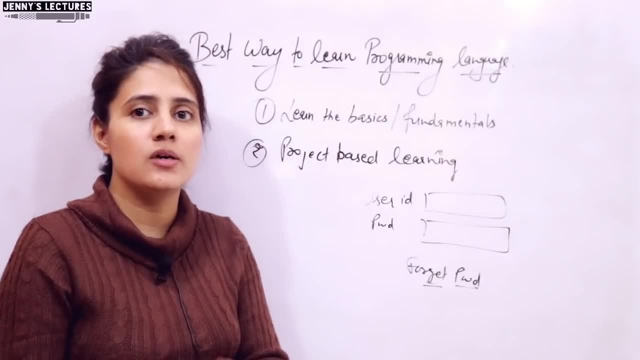 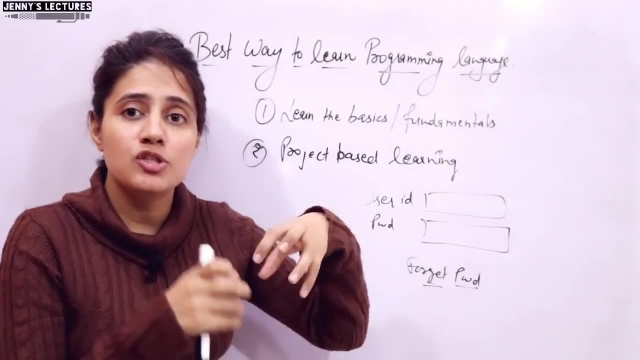 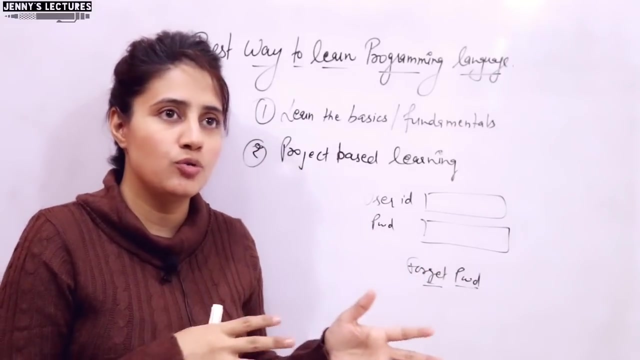 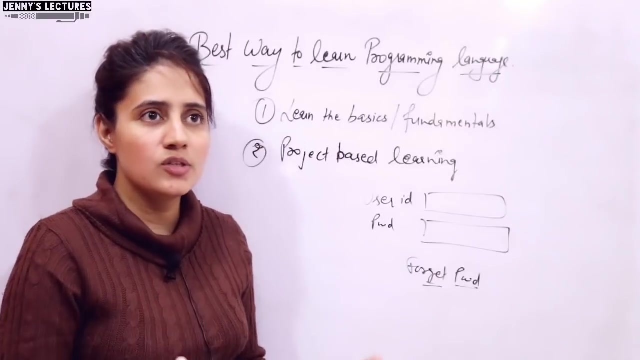 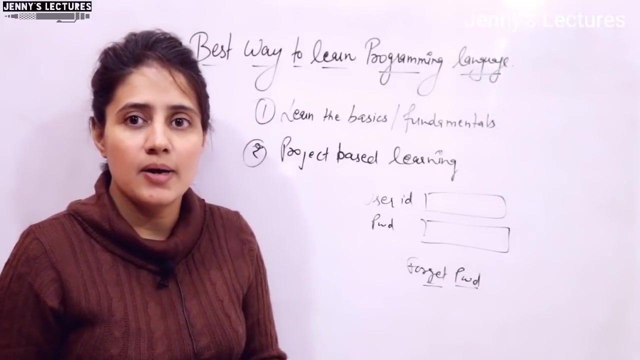 remember, sooner you start playing with the code, the faster you will learn that concept. and this is true, so that only apply for slept. so let's see. let's take one more example, that example of time complexity. this is, i think you know, optimization of algorithm. you have to write optimized algorithm, like the time complexity. 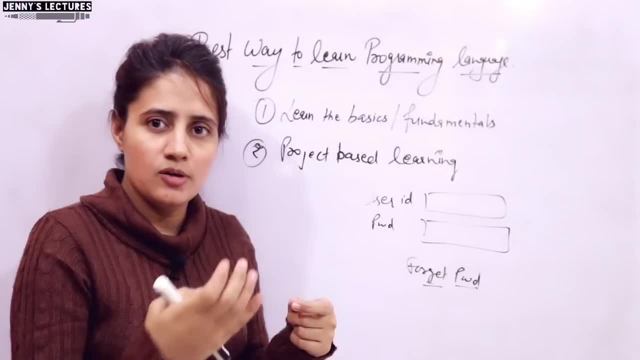 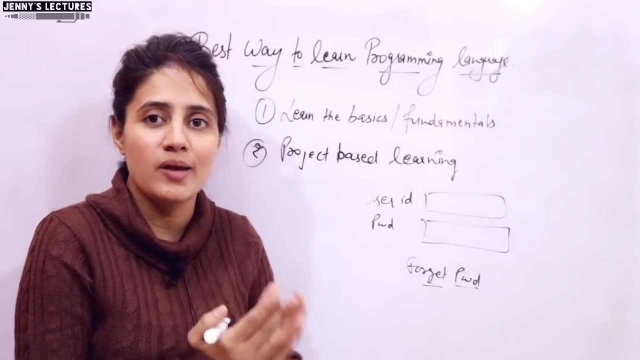 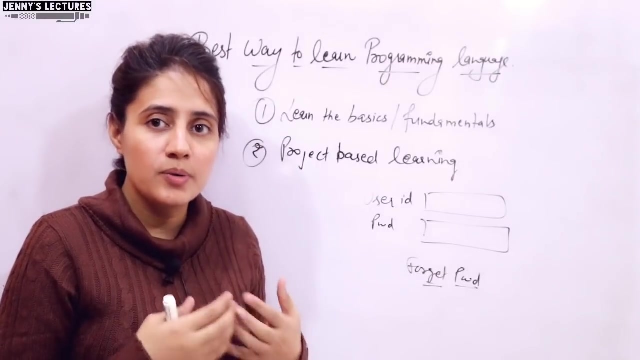 in within that app and it is taking 10 seconds to load. so it is not good. you think that how can you reduce this time? at that time, the actual meaning of time complexity, the actual meaning of optimization of algorithm will, you will understand how to optimize and why you are optimizing your algorithm. because if 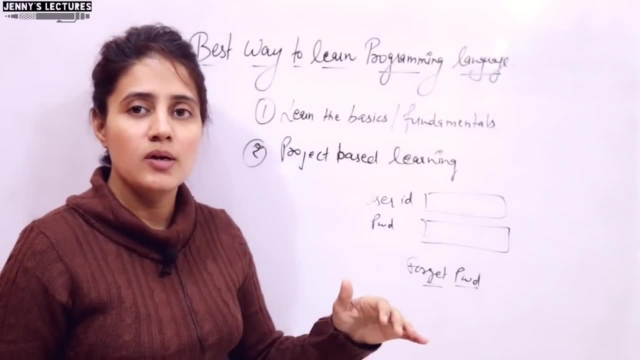 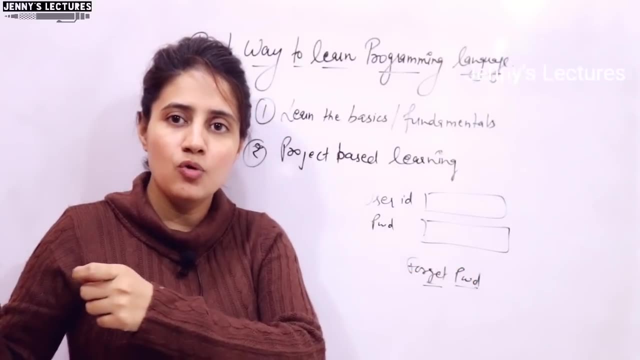 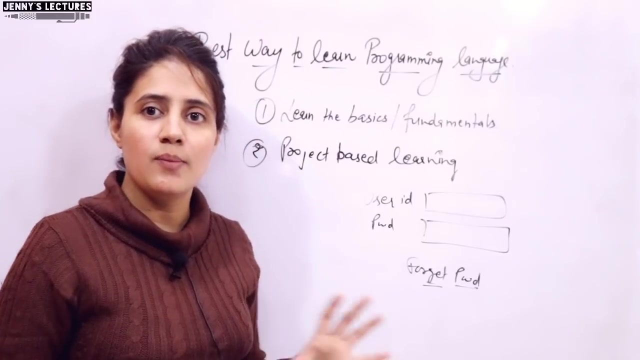 anything is taking 10 seconds to upload, then and some other things, some other wrap is taking only one second to second, then definitely the users will go for that app that is taking less time. so you have to optimize your code also, right, so at that time you will come to know the meaning of these things when you are. 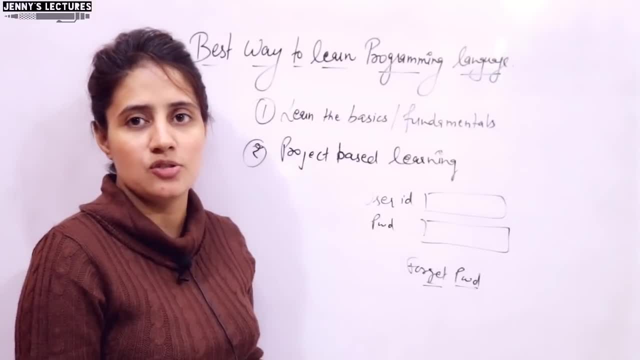 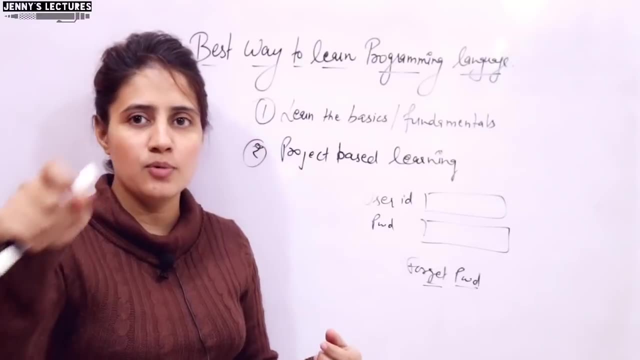 working on projects, when you are making apps, when you are making any applications, any software's. so, rather than searching how to learn a language, like how to learn Java, Java tutorials, watching those tutorials, just writing programs. no, that is not enough, it is not right path. start making a project. 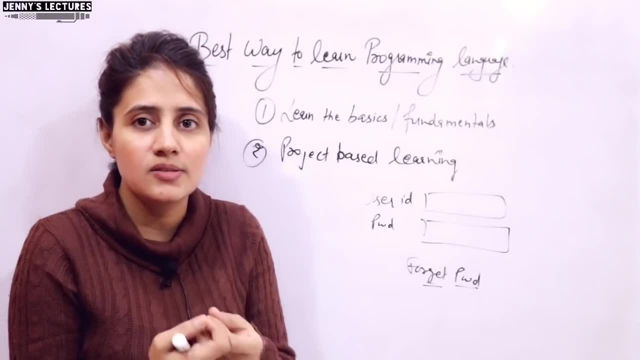 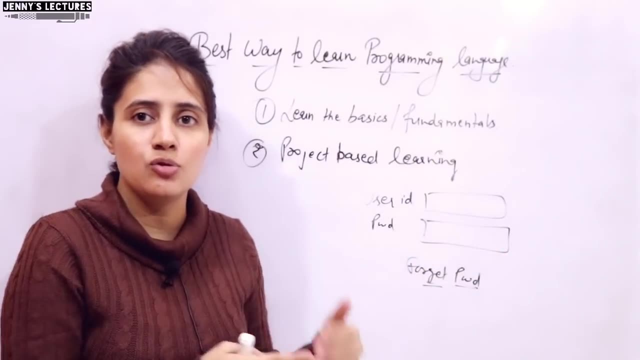 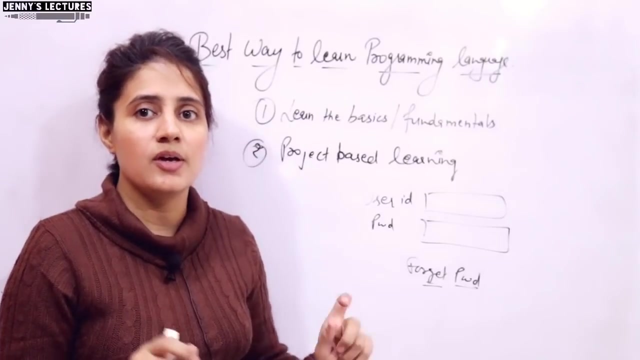 if you stuck somewhere, then search how to implement this thing in project, how to implement this thing using java or any language. then you will come to know, then the solution will come. many solutions maybe will come when you are searching and see. please do not underestimate the power of search. unlimited resources are there on internet. you just have to search. 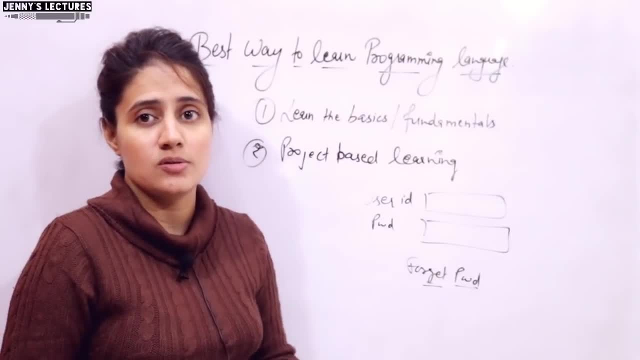 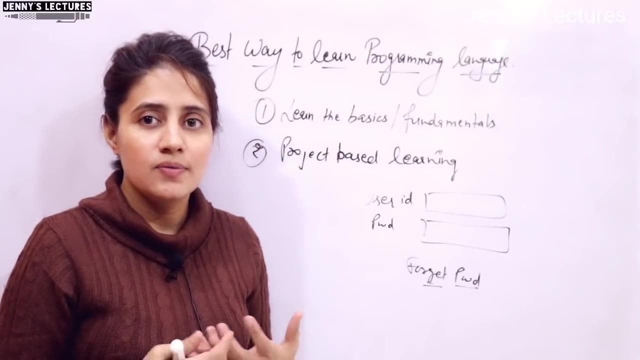 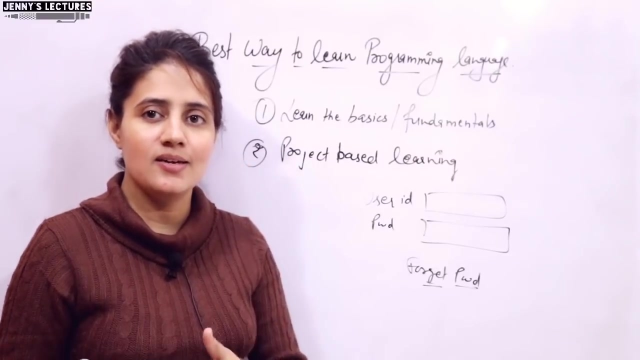 those resources. you just have to utilize those resources. please do not be dependent on just on your books and the faculties and on your college self-learning. this is also very important and i guess you will learn more by applying this technique, this self-learning techniques, rather than depending on your faculties, on your college and your textbooks. right, so start building a.